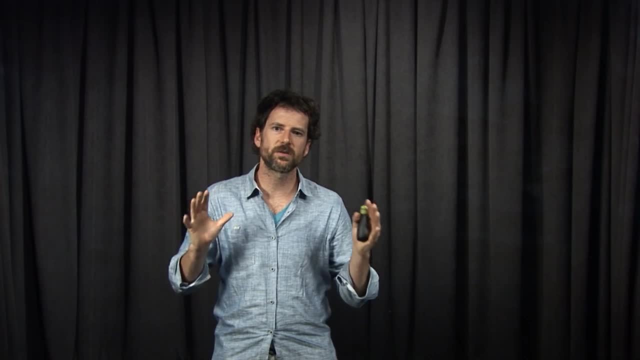 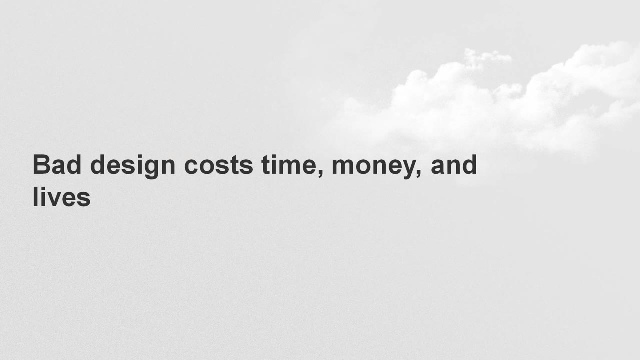 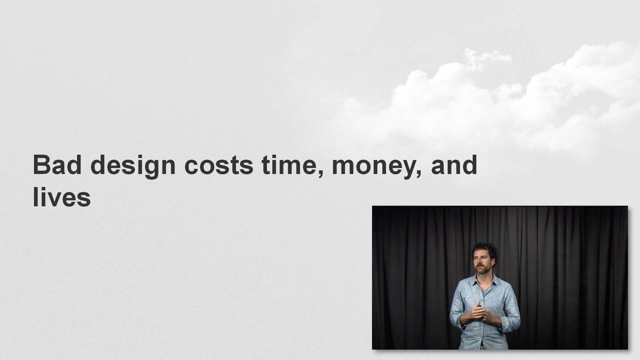 put computing on hundreds of millions of desks, enabling us to do things like create documents and share photos, interact with family and find information. Conversely, bad design costs time, money and lives. Medical devices, airplane accidents and nuclear disasters are just. 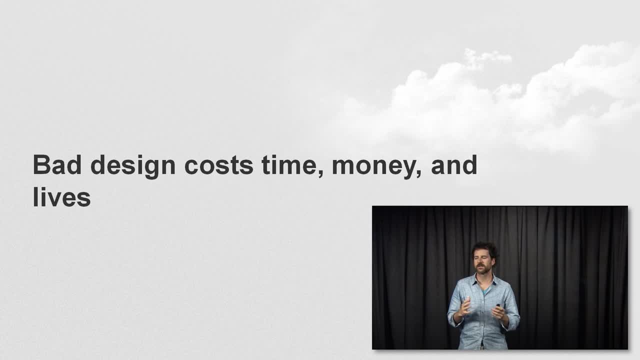 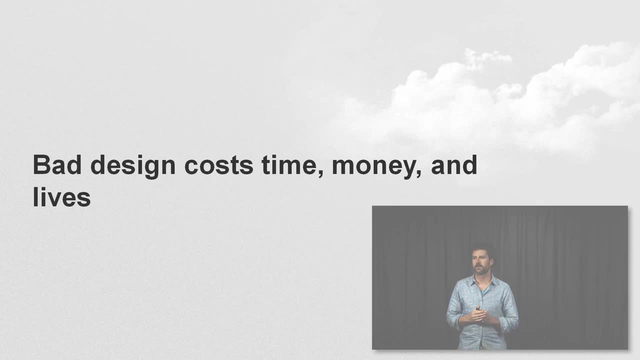 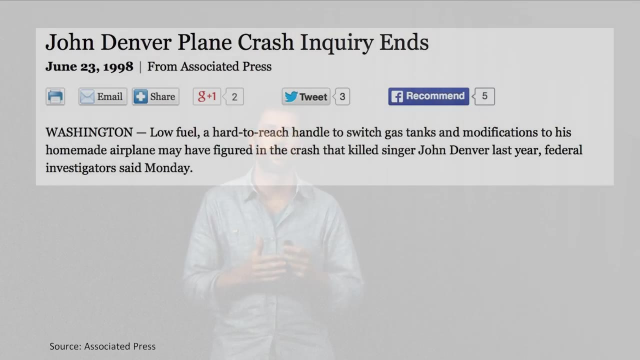 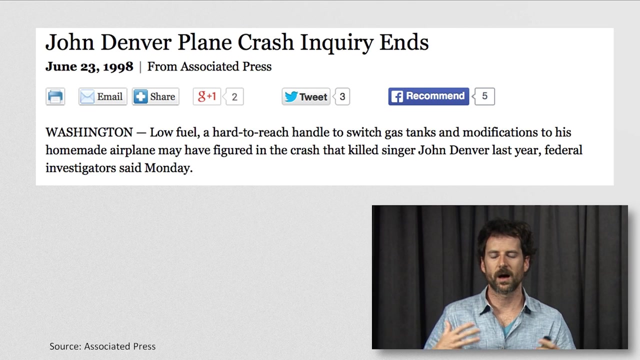 a few domains where bad user interfaces have caused serious injury, even deaths. What gets me is that many of these interface problems could have been easily avoided. Fixing these problems requires following just some basic principles like consistency and feedback. Growing up, I loved John Denver's music. In 1998, he passed away tragically while flying. 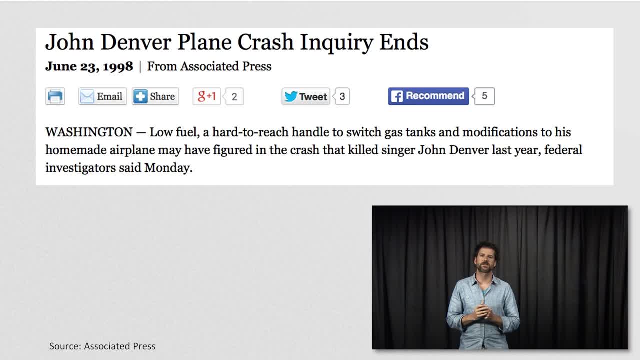 his airplane. As is common in situations like this, there were a number of factors in play. Usually, deaths mean that multiple different bad things happen simultaneously, one you can usually recover from. In John Denver's case, it was a combination of low fuel, a 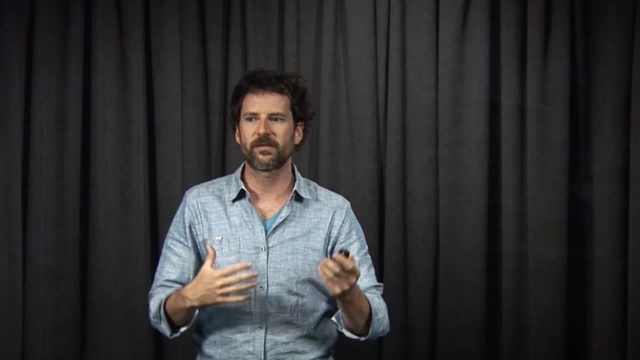 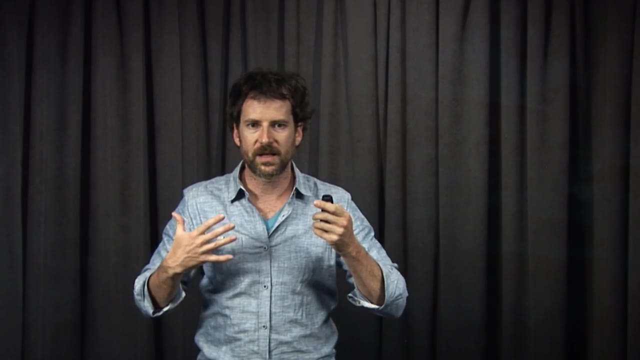 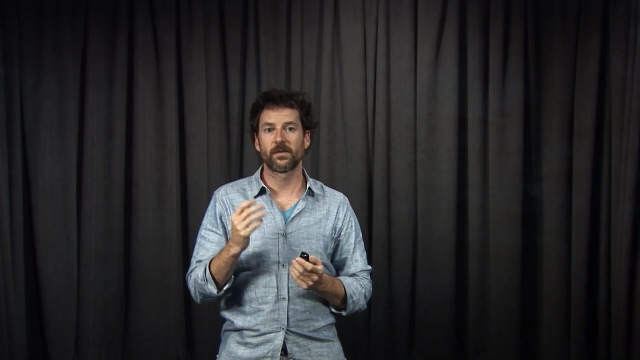 hard-to-reach handle to switch the gas tanks and some custom modifications to his plane. This meant that a bad user interface required John Denver to turn around and the ergonomics of the cockpit actually contributed to his death. Here's another remarkable example of an emergency telephone where you're supposed to dial 999.. 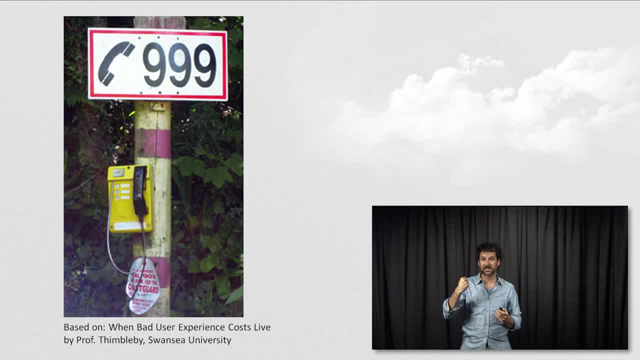 However, the physical telephone itself only has the numbers 1,, 2, and 3, and so there's a post-it note at the bottom. We'll get to that later as a key signal of bad design. It explains how to map a bad design and how to map a bad design and how to map a bad. 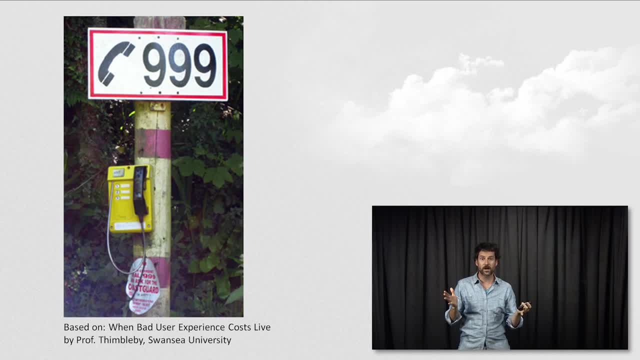 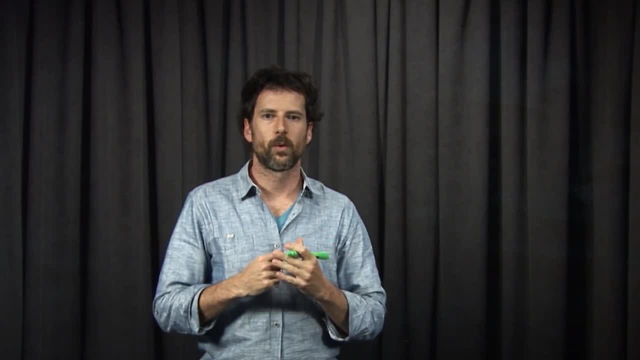 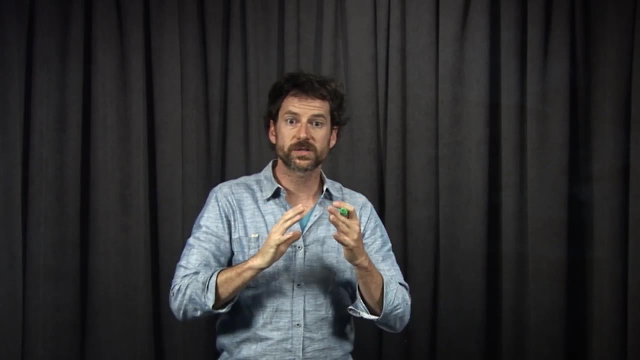 design and the buttons available to the number that you need to dial Crazy. But it's not just the dramatic reasons that good design can be so transformative. We interact with hundreds of websites, apps, ticket kiosks, all sorts of physical, digital and combined.